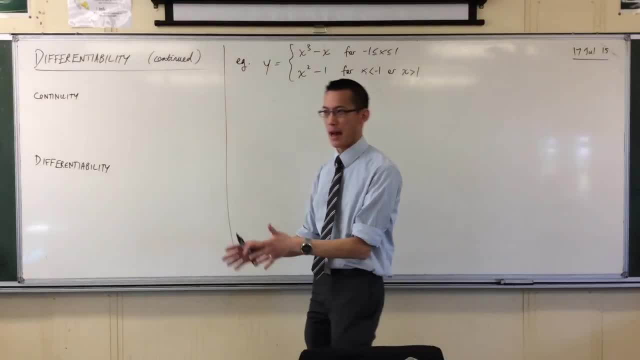 Right now. what we're going to do is we're going to be a little more formal about it. I try as much as possible not to start with formal definitions, because you get lost in all the notation and that kind of thing. But now that you get the idea, it's time to get the symbols on the paper. 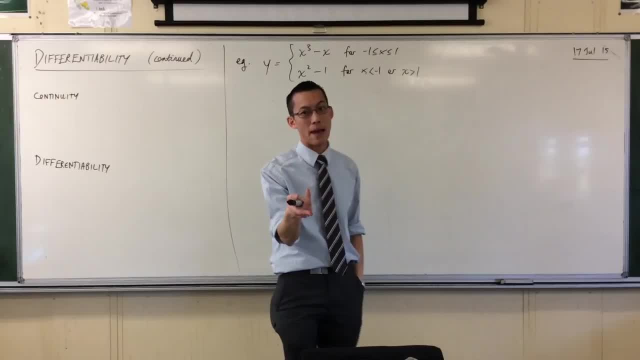 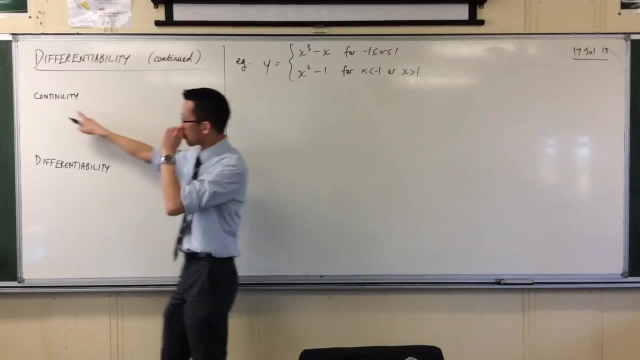 So I want you to think back to this. You can probably find it in your paper, but I want us to write it up again anyway, because it's worth seeing the parallel between these things If I want continuity for some function at a certain point. 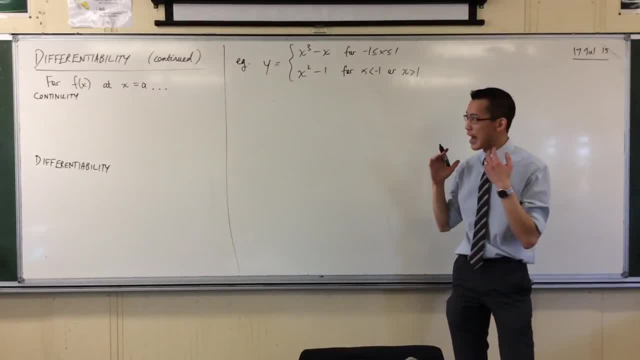 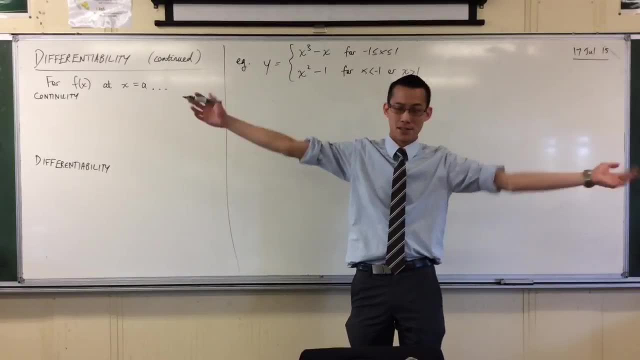 If I have a function and I'm thinking about whether it has continuity or not, I want continuity or differentiability at that point, Because we've seen there are functions which can be continuous- a whole bunch of places- and differentiable- a whole bunch of places. 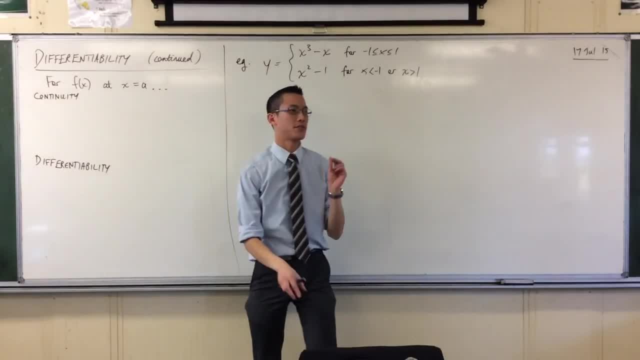 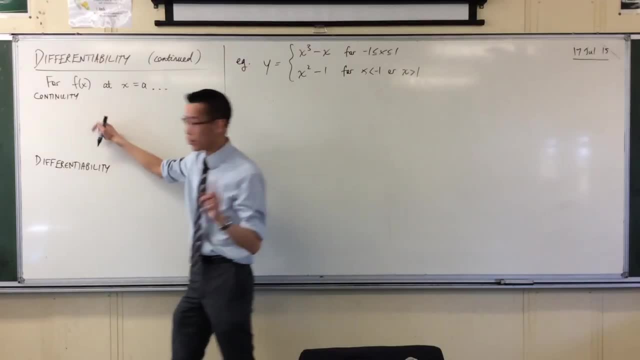 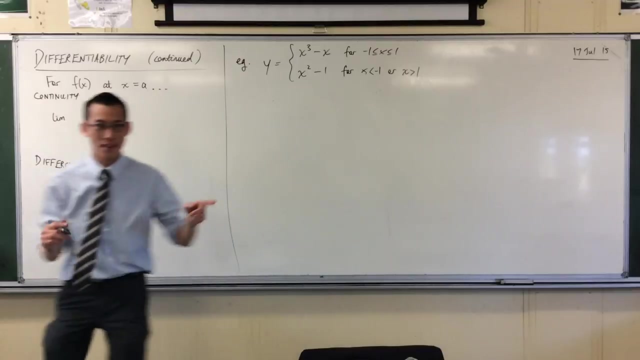 But they're just particular critical points when you really have to inspect these carefully. Formally speaking, what would it mean to be continuous? And I'll give you a clue: It starts with a limit, Anyone remember? Yeah, Minsoo. 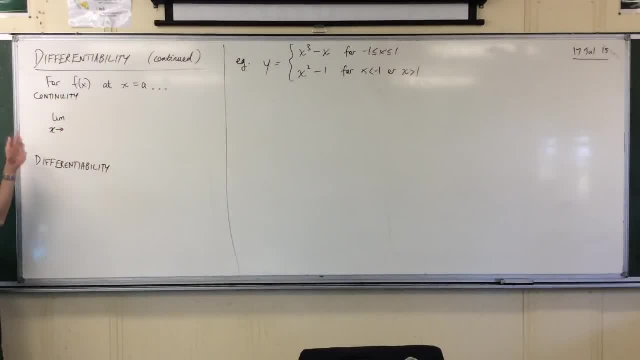 Positive, Ah, very good. So here's what's happening. We want to think about this certain point. We want to get closer and closer. that's what the limit's about to that point. But, thank you, Doris, we need to look carefully at what happens from one direction versus the other. 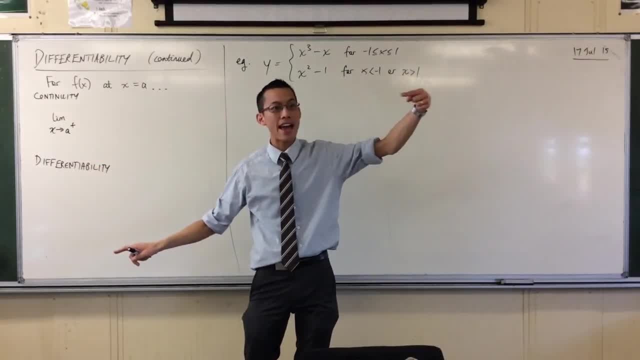 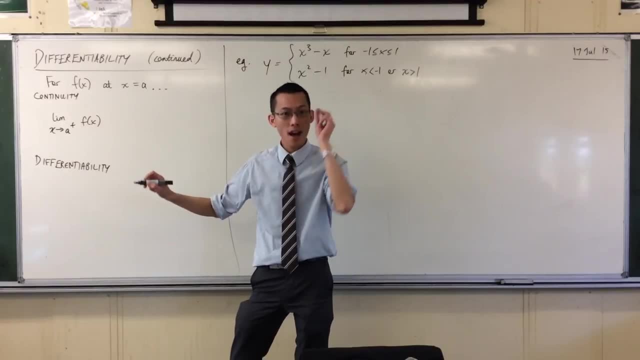 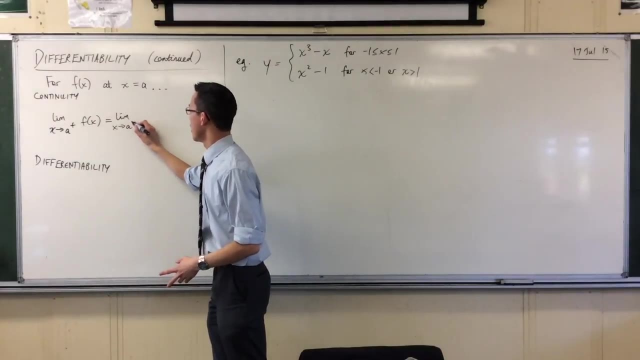 So a plus means come from higher values, that's, from the right, And I want to know what's happening to f of x. I want that to be doing exactly the same thing as what happens if I approach, but from the opposite direction. 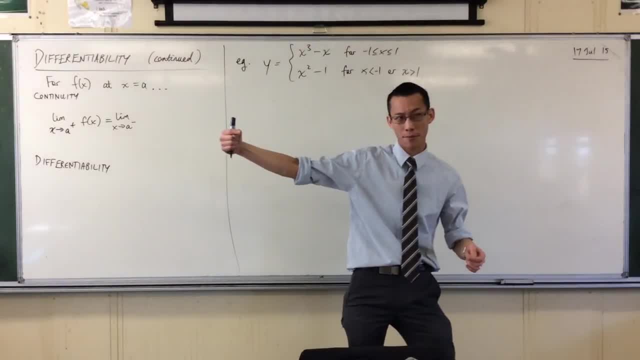 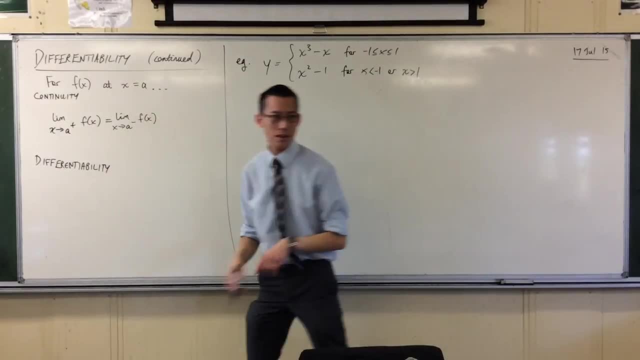 So a with minus means come from lower values come from below. so that's from left to right. We want to see what's happening to f of x from that direction, And both of those should also be equal to a third thing, do you remember?